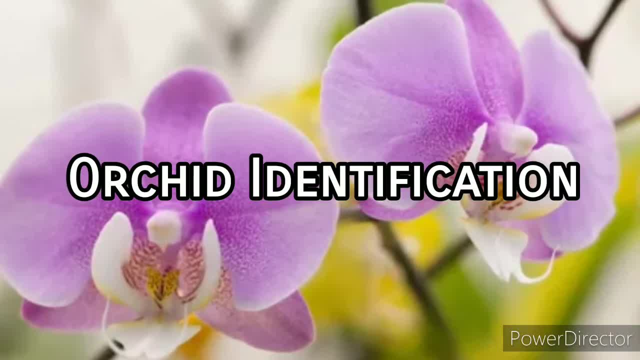 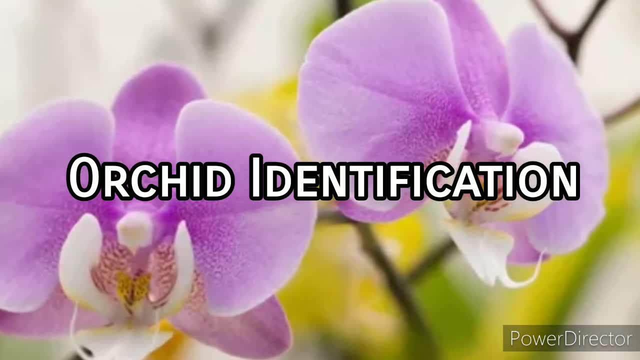 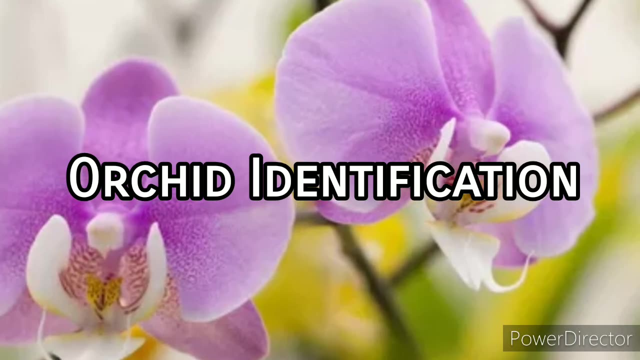 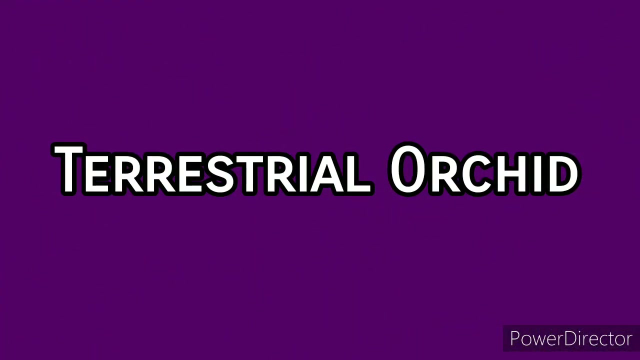 Hi, welcome back to whimsy crafter. I hope you all are doing great. We often buy orchids without knowing about their care routine and their type, So in today's video I'll be discussing the basic orchid identification so that you can better care for your orchids. When we talk about orchids, there are basically two types of orchids. The first type is the terrestrial orchid and the second type is the epiphytic orchid. When I 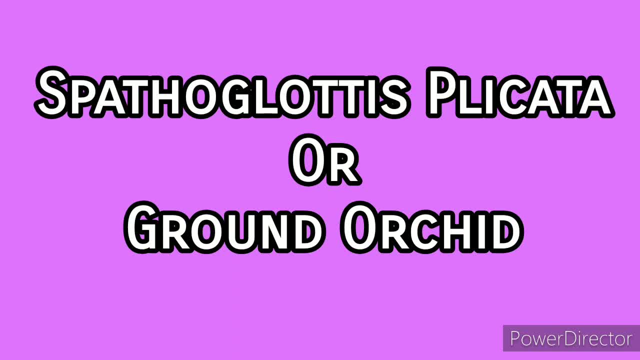 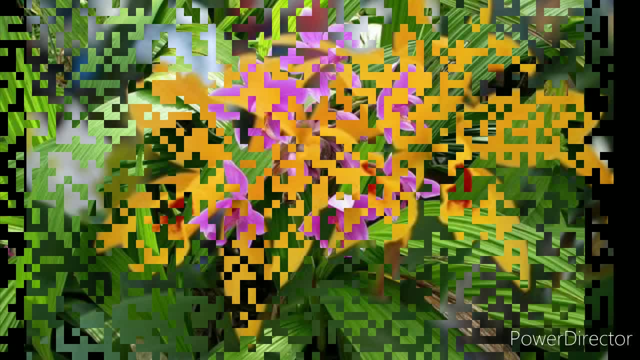 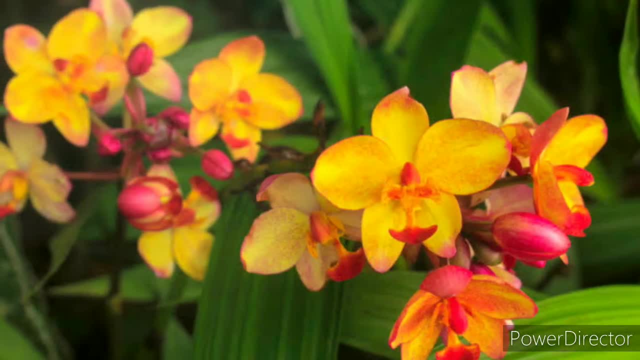 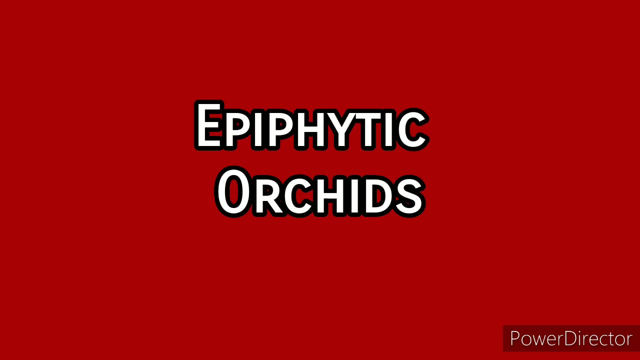 talk of terrestrial orchids, I mean spathoglottis plicata or ground orchid. This is what ground orchids look like. There are multiple colors in which they are available. They are usually grown in the same type of media in which houseplants are grown, and they like moist, warm conditions and filtered light. The next type of orchids is epiphytic orchids. Epiphytic orchids grow on trees and crevices of rocks, but they are not parasitic. 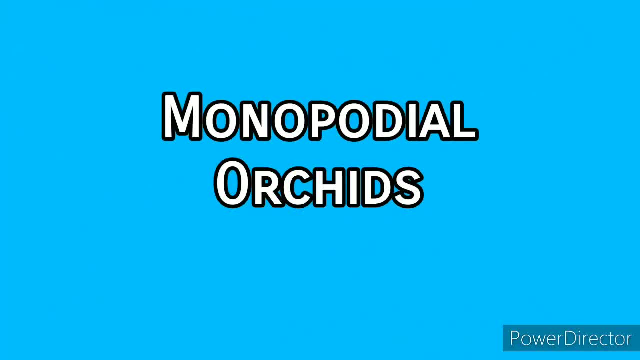 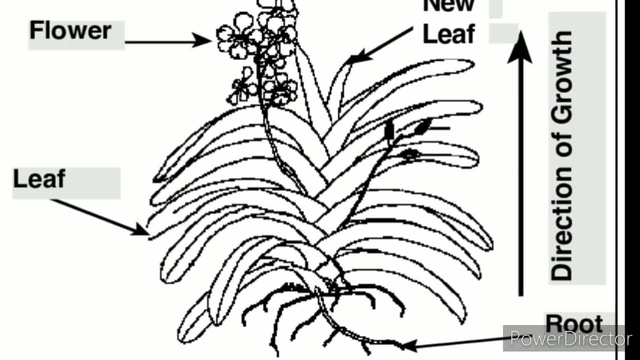 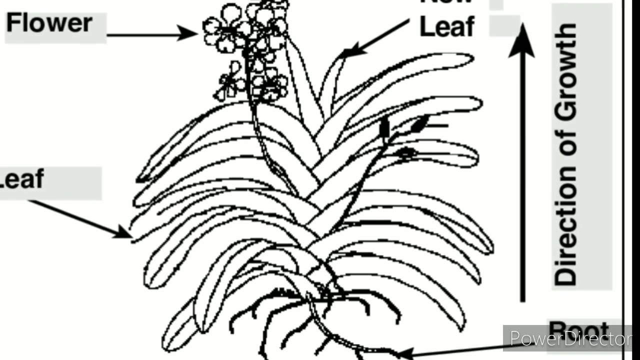 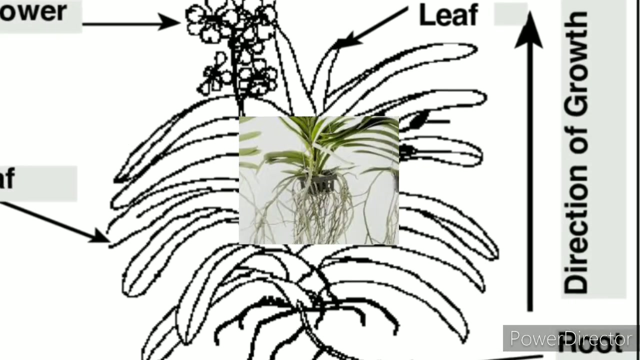 plants in the sense that they don't derive nutrition from the host. Now they can be further classified into monopodial orchids, And by monopodial orchids I mean this diagram. Look at the diagram. There is a central axis on either side of which leaves emerge and the flower spikes emerge from in between the leaves. This type of orchid has no mechanism for storing water, So 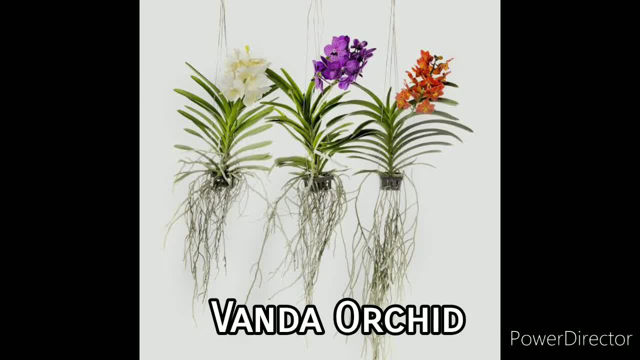 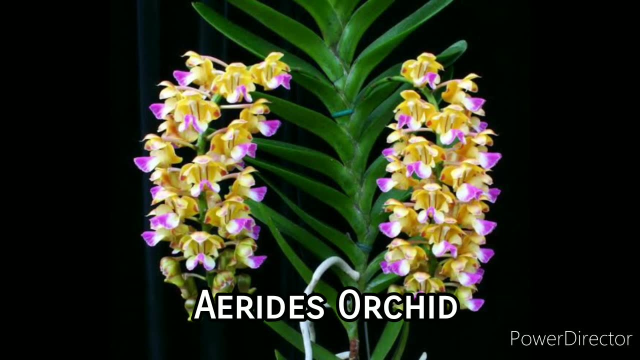 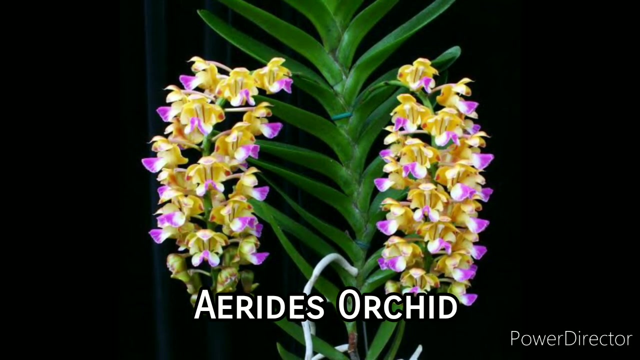 some common examples of monopodial orchids include Vanda orchid, like you can see over here in the picture, And you can see that there is a single central axis on the either side of which leaves are growing. The second example of monopodial orchids is the Erides orchid And I would like to mention that monopodial orchids are high light loving orchids And I'm showing you the orchids in the. you know downward graduation of light. So if you 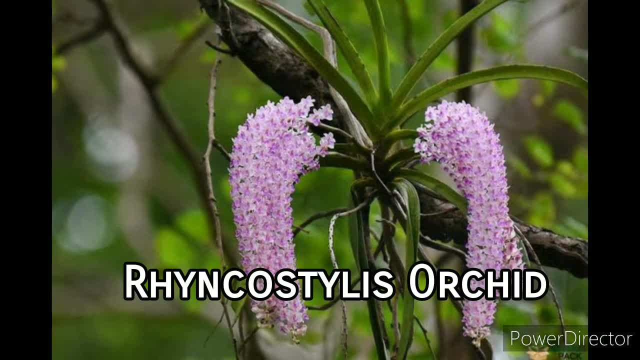 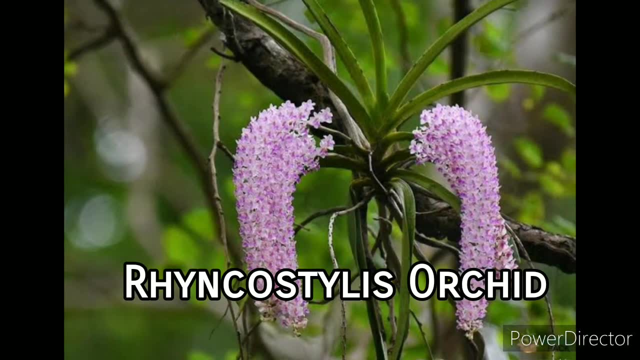 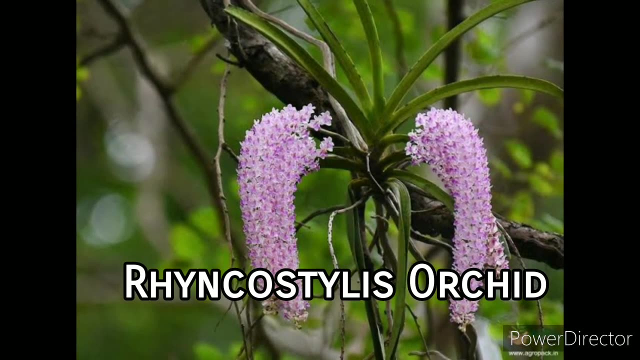 requirement. The third type of monopodial orchid is the rincostylus orchid. All these type of orchids require high moisture and light conditions, but by light I mean filtered sunlight, not direct sunlight. The fourth type of monopodial orchid is obviously our phalaenopsis orchid. They have 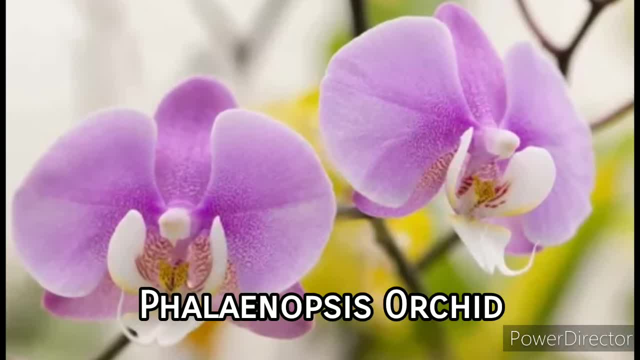 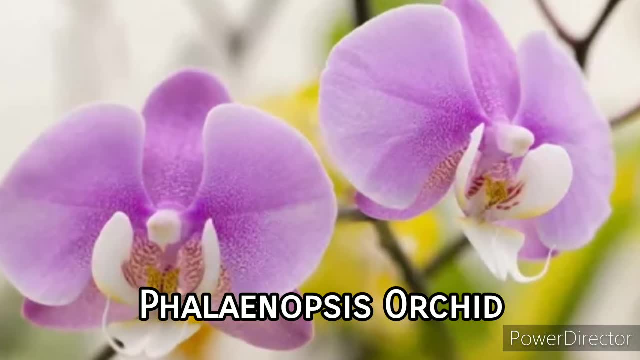 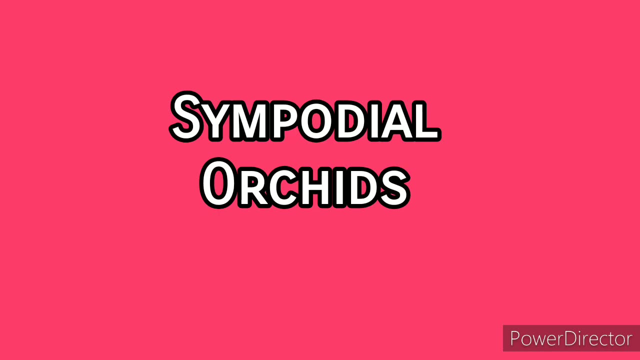 beautiful spikes which remain for 45 to 60 days on end, but their temperature and light requirements are comparatively lower than the previous three monopodial orchids that I showed you. They can be easily kept indoors. The second type of epiphytic orchids are sympodial orchids, like the diagram. 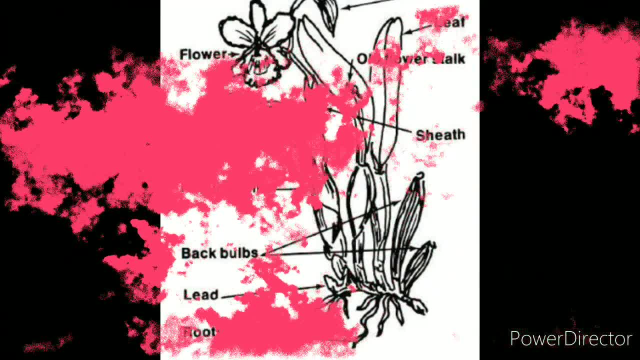 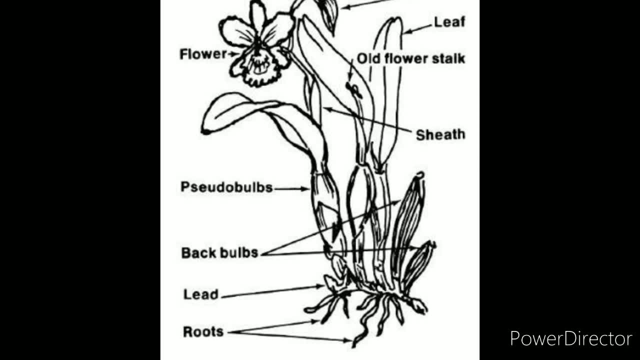 that I'm going to show you right after this. If you take a look at this diagram, you'll see multiple growths growing from the base, And they are usually in the form of bulbs and pseudobulbs, and then there are leaves, and then there are. 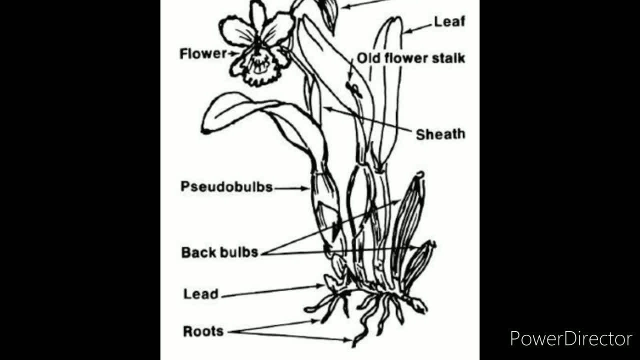 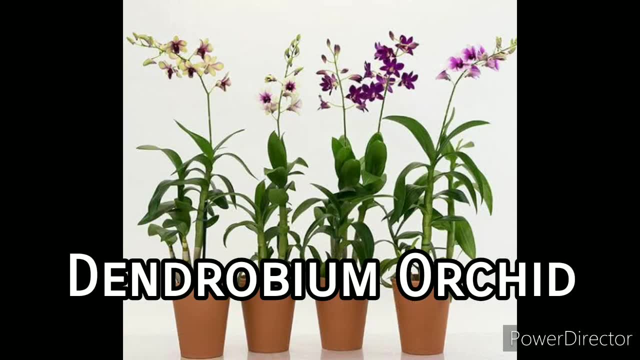 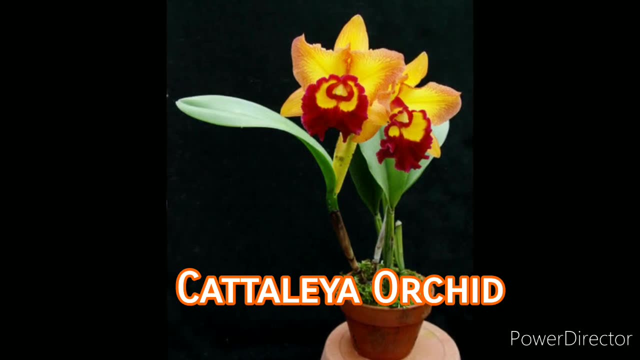 spikes that emerge from in between the leaves. Some very common examples of sympodial orchids include your dendrobium orchids, the most popular ones, the beginner's orchid as we know it. The next kind of sympodial orchid is obviously cattleya orchid with large showy. you know flowers in. 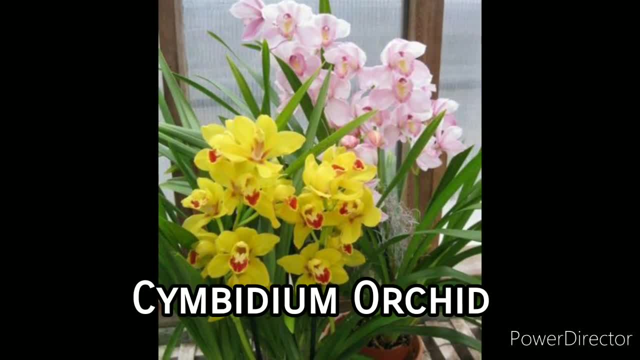 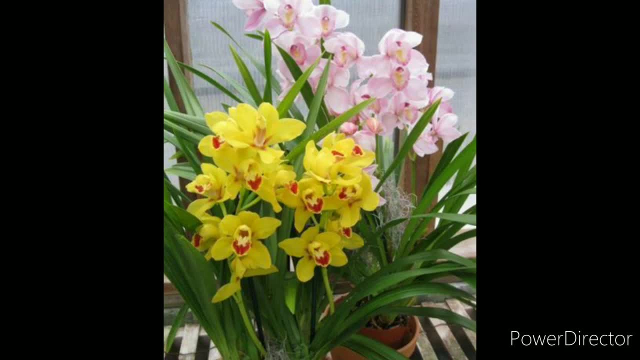 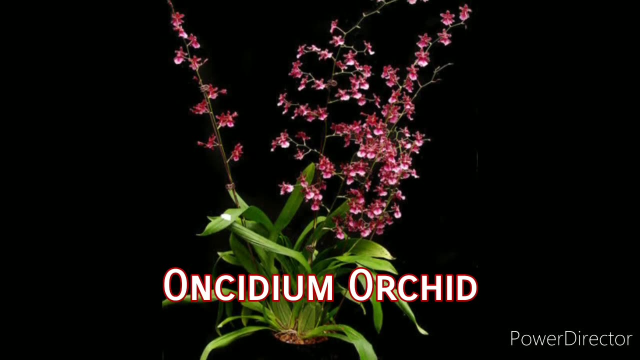 various colors and hues. The third kind of sympodial orchid is the cymbidium orchid. All of these have mechanisms to store moisture in them in the form of pseudobulbs. The fourth kind of sympodial orchid is our oncidium. 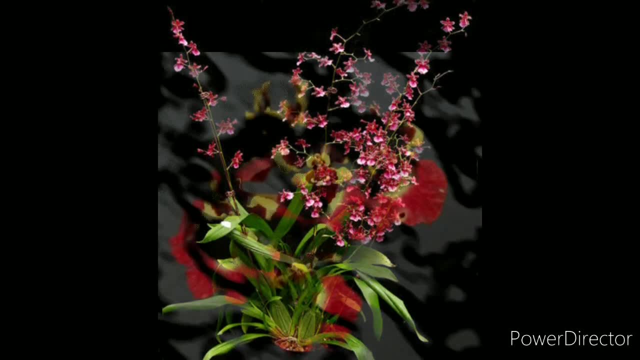 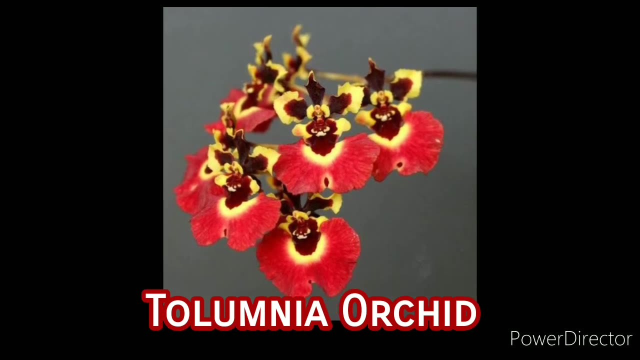 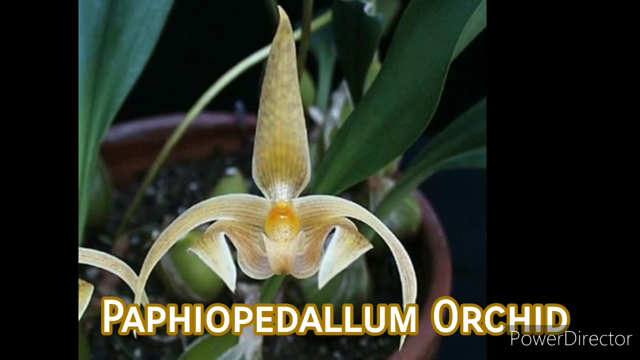 orchid. Another subtype of oncidium orchid is the tulumnia orchid. All of these sympodial orchids are moderate light loving plants. The next type of sympodial orchids that we have is pafeopedilum. This is a moderately low light. 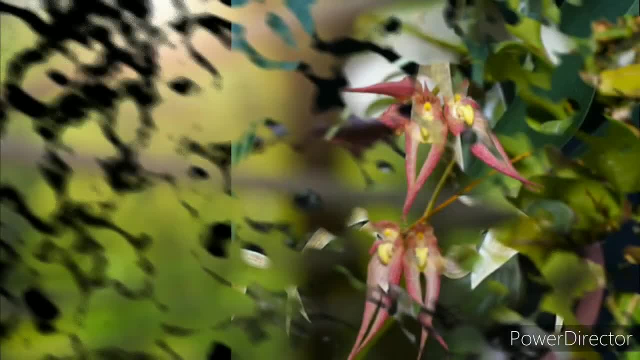 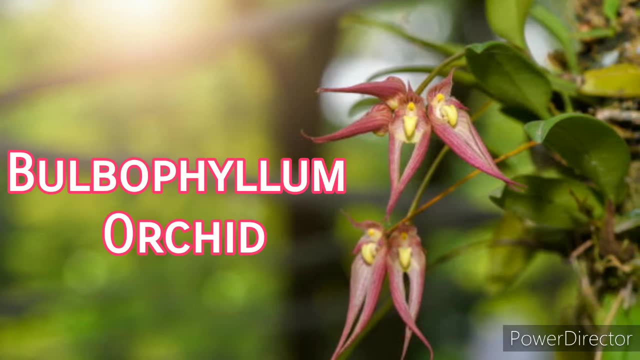 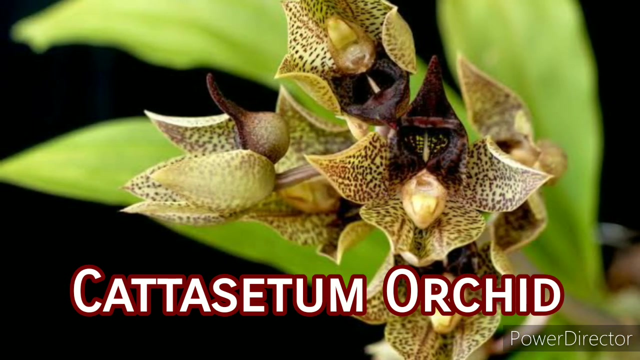 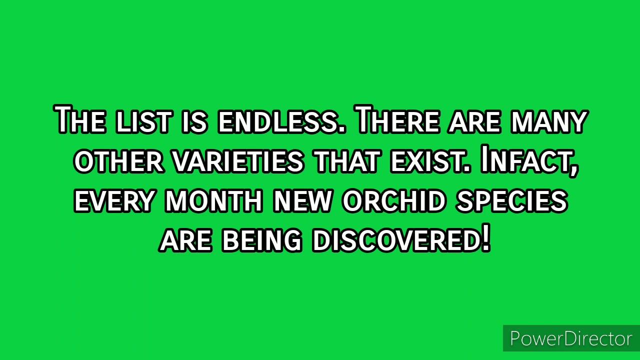 loving orchid usually found at the forest floors. Another such example of low light loving sympodial orchid is bulbophyllum orchid. Catasetum orchid is yet another type of sympodial orchid. So I have tried to provide a brief overview of the basic kinds of orchids, but this is not all the